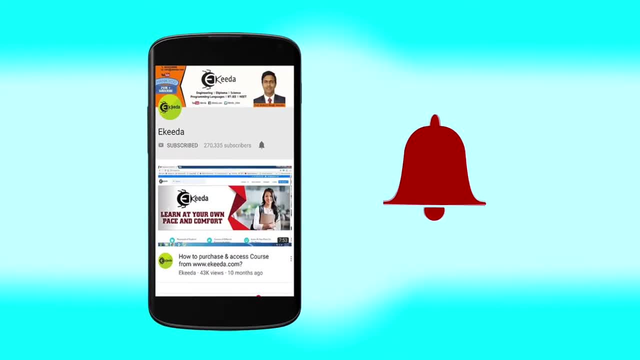 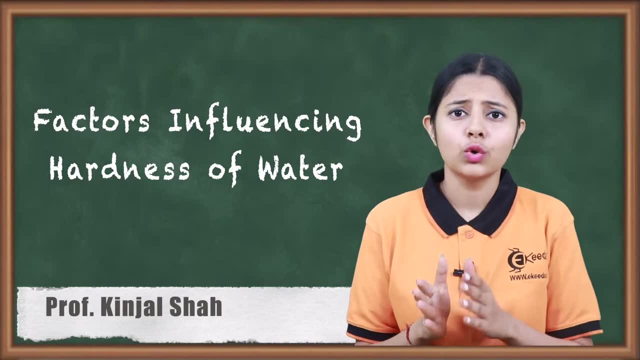 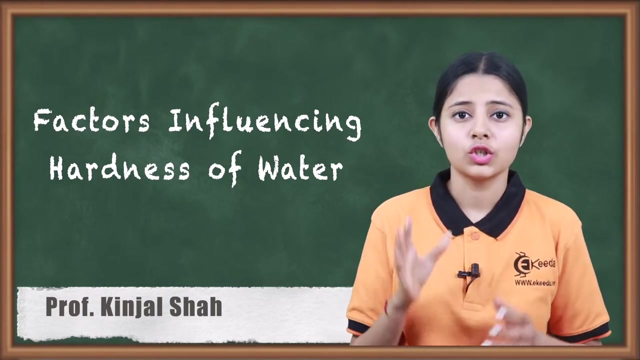 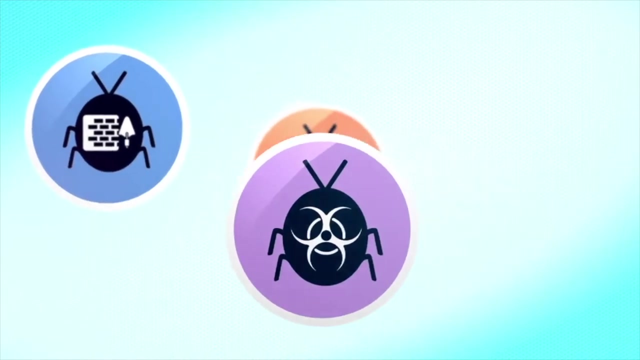 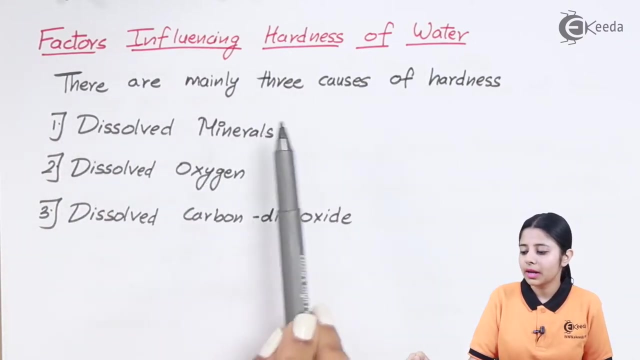 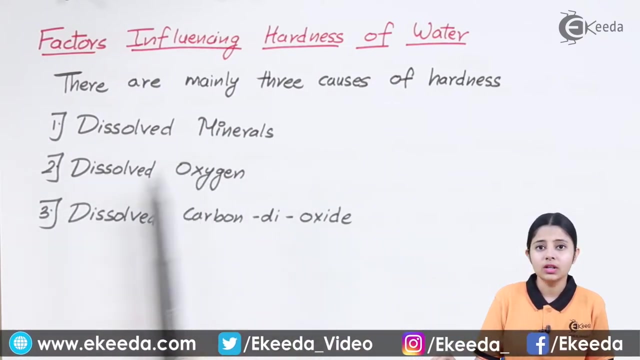 Click the bell icon to get latest videos from eKIDA. Factors influencing hardness of water. There are three main factors. Those are dissolved minerals, dissolved oxygen and dissolved carbon dioxide. Dissolved minerals are all the minerals which are present in the water in the form of salts. That means these minerals, they 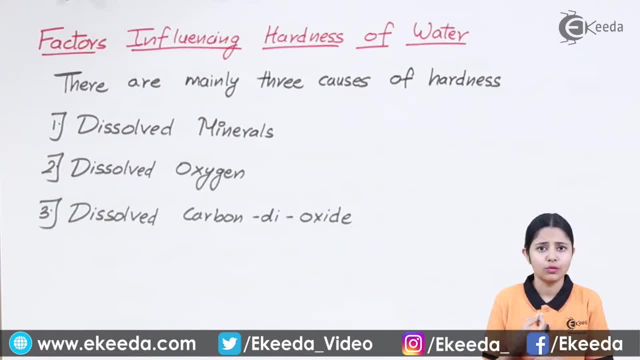 can be heavy metal, which can be mixed with some other things like sulfates or chlorides, and make salts of them, And these salts are dissolved salts and are dissolved in water. Because of that, the dissolved minerals make the water hard. The second one is dissolved. 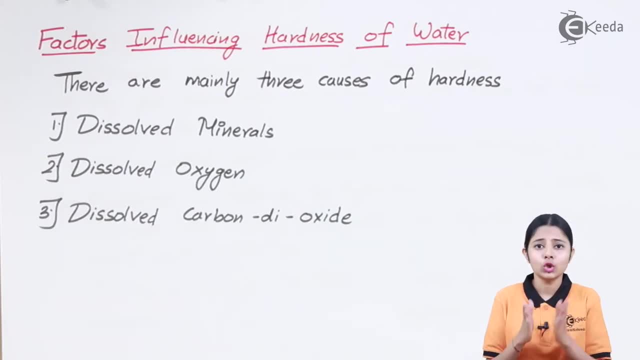 oxygen. Dissolved oxygen is a tricky one. Why? Because H2O is water, Water itself contains oxygen, and that oxygen is in the dissolved form. The dissolved oxygen does not make the water hard, But this dissolved oxygen reacts with many minerals and because of that it 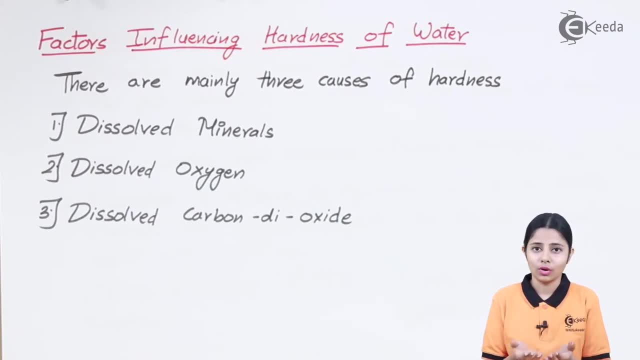 makes different oxidation products which make the water hard water, And the last one is dissolved carbon dioxide. Dissolved carbon dioxide is a mineral which is present in the water. It is not very desirable in hard water And that is the reason why when we convert, 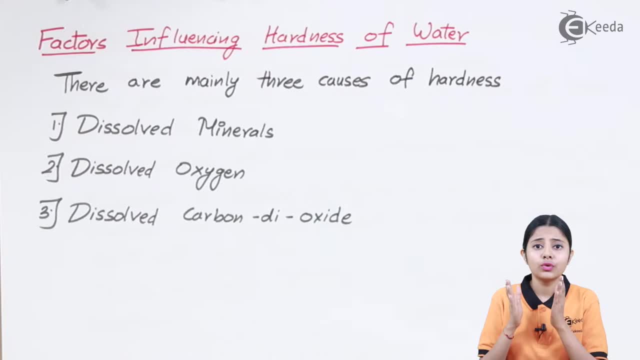 hard water into soft water to different procedures. we have a different chamber or a different procedure for just removing the dissolved carbon dioxide, which is the last step of converting the hardness of the water into the softness of water. Dissolved minerals. Dissolved minerals. 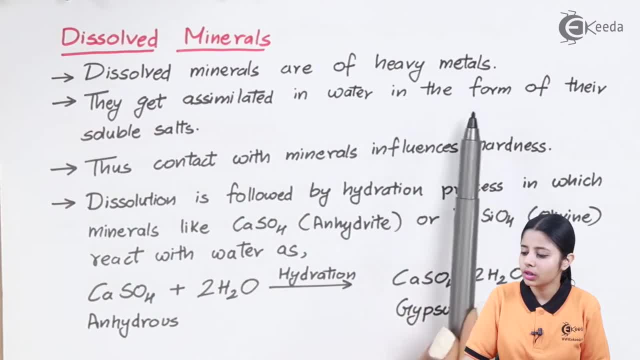 are of heavy metals. They get assimilated in water in the form of the soluble salts. So there are many minerals. there are many metals like lead, sodium and more other metals like lead, But these metals are not soluble in water. They get soluble in water once they 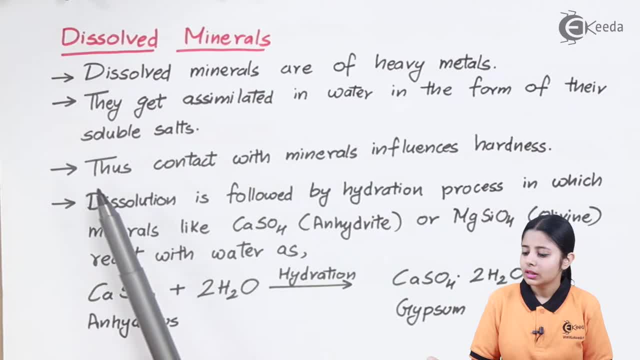 form salts of it. Let us see how they form salts of it. Thus, contact with minerals influences hardness. Dissolution are followed by hydration process, in which minerals like CaSO4, which are also known as anhydrides, or MgSiO4, also known as Olarin, react with water as So now. 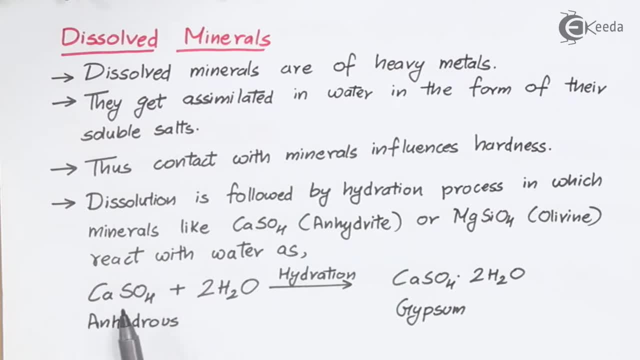 I have anhydrides CaSO4. This CaSO4 anhydrides is not soluble in water right now, But once I have anhydrides CaSO4 in my water, that is 2H2O. this process is known as hydration. 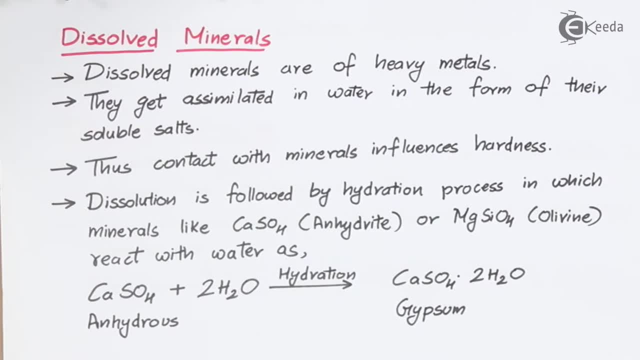 Hydration is a type of chemical reaction wherein the water clings with my reactant 1.. That means over here my reactant 1 is CaSO4, reactant 2 is water, But when I see the product it is CaSO4.H2O. This process is known as hydration and this .2H2O is known as water of crystallization. 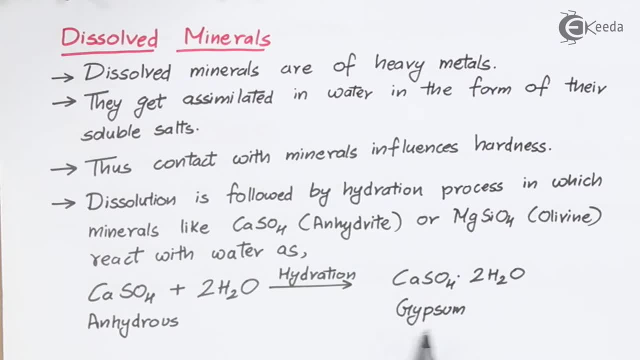 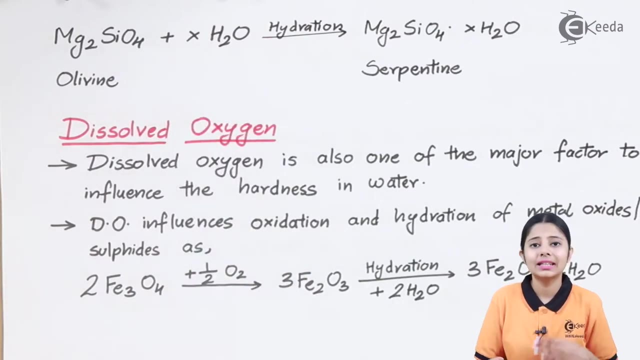 This water of crystallization helps CaSO4 form gypsum, which is a soluble salt, and this soluble salt of anhydrides, CaSO4, gets dissolved in water and thus makes pure water as hard water. Now I have Mg2SiO4 plus XH2O Over here. this X means any number of H2O, Depending. 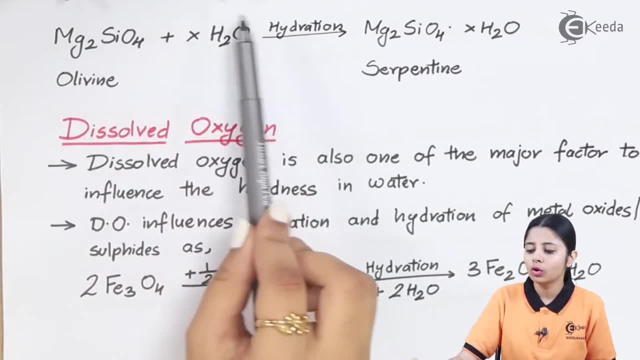 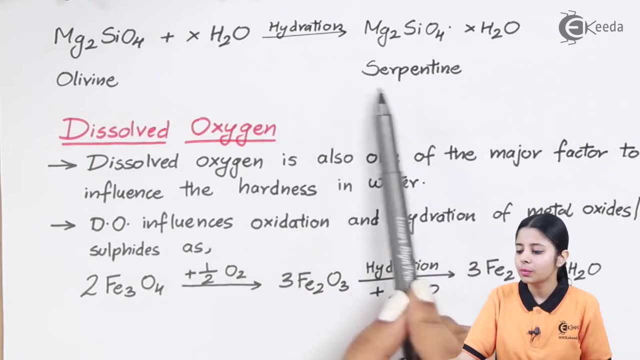 upon what kind of Olarin I have, I will need the amount of H2O Now. this also is the process of hydration, forming Mg2SiO4.XH2O, which forms a serpentine, and this serpentine is soluble in water. Next is due to my dehydration process, I have anhydrides. CaSO4.H2O is known as water. 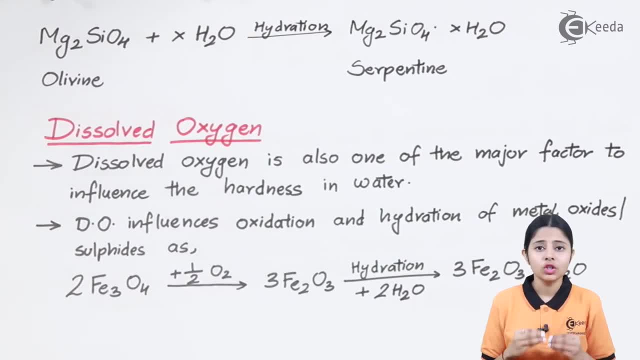 Next is due to my dissolved oxygen. as I said, dissolved oxygen itself does not lead to hardness of water, but this dissolved oxygen oxidizes certain minerals. that means it leads into the oxidation reaction with certain minerals and this reaction gives products which are now soluble in water, and these products are nothing but impurities which are soluble in. 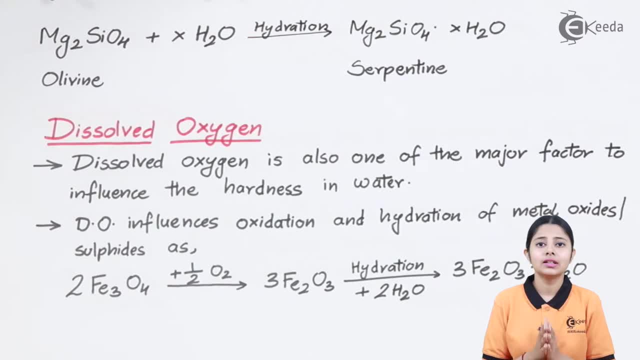 water, and that makes the pure water as hard water. Let us see the different reactions through which it happens. Dissolved oxygen is also one of the major factors to influence the hardness of water. Dissolved oxygen is also known as DO. So when you are reading or when you are writing, DO. 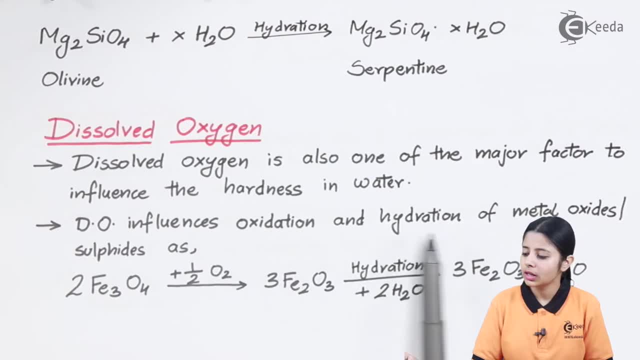 can also be written as dissolved oxygen. Influences, oxidation and hydration of metal oxides, sulphides, as follows. So over here I have 2Fe3O4 in presence of half O2 instead of half O2. you can also write nascent oxygen, but nascent oxygen is unstable and that is the reason. 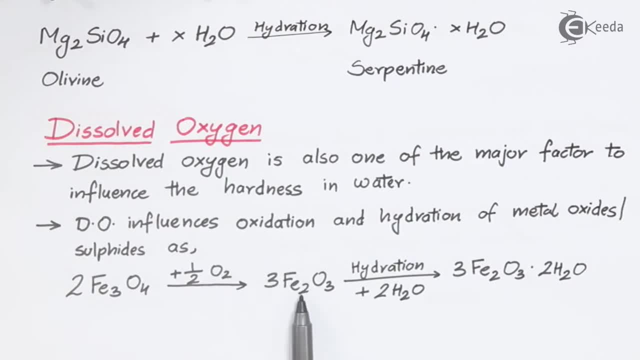 why we have written over here half O2 forming 3Fe2O3.. Let us see the balancing of this part of the equation over here. So 2Fe3O4. let us just have a look at Fe. I have 3 into 2, that is, 6Fe on the reactant. 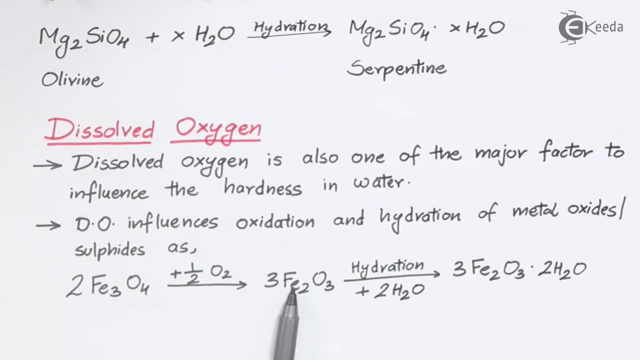 side. on the product side also, I have 3 into 2, that is 6Fe. Let us look at the number of oxygens now: O4 twice 2Fe3O4, right so O4 and twice so 4. twos are 8 plus half O2, half. 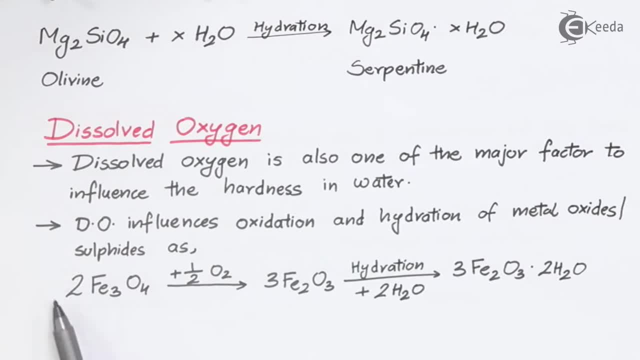 O2 is 1 oxygen, so 8 plus 1 is 9 on my reactant side. let us see the product side: 3 into 3, that is 9.. So 2Fe3O4 is equal to half O2 plus half O3 into 3.. 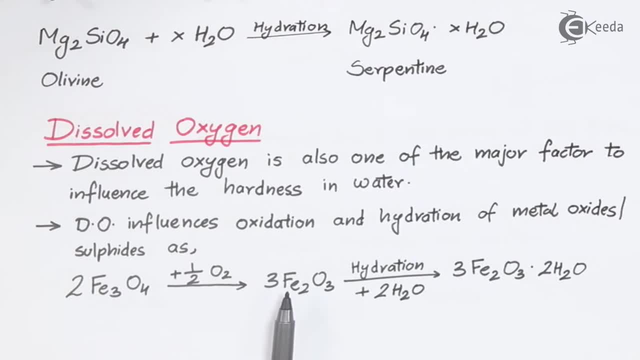 So this 2Fe3O3 plus half O2 forming 3Fe3O3 is a balanced reaction and this reaction is known as the oxidation reaction. Oxidation reaction is nothing but addition of oxygen over here on my reactant side I had 8.. 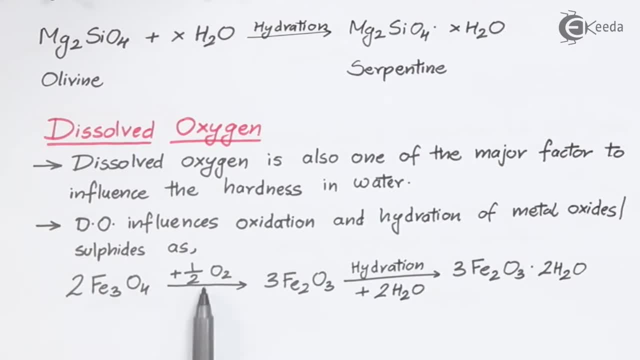 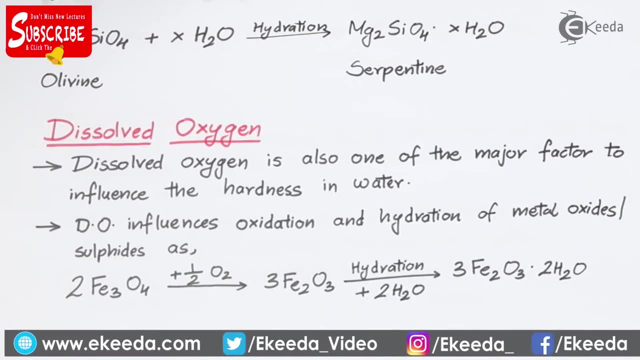 So over here on my reactant side I had 8, plus I added 1, so on the product side now I have 9.. Moving on is my hydration reaction. Hydration reaction is nothing but addition of water, addition of H2O molecules. So whatever my reactant is, plus 2H2O forming in the product. 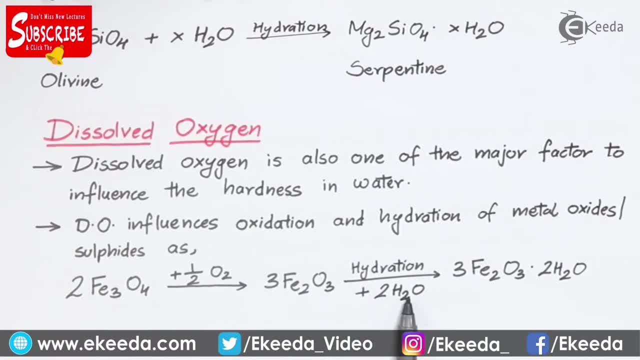 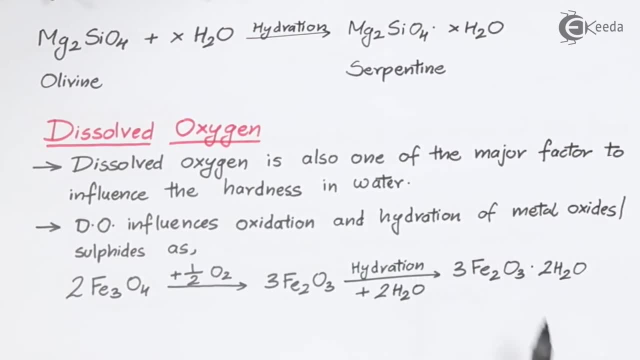 to O. So, whatever my reactant is, just add n molecules of water, whatever is needed for that particular reactant, and that becomes the water of crystallization, and this itself becomes a salt, and this salt is now soluble in water. Now, hence, we proved that because of oxygen which is present, 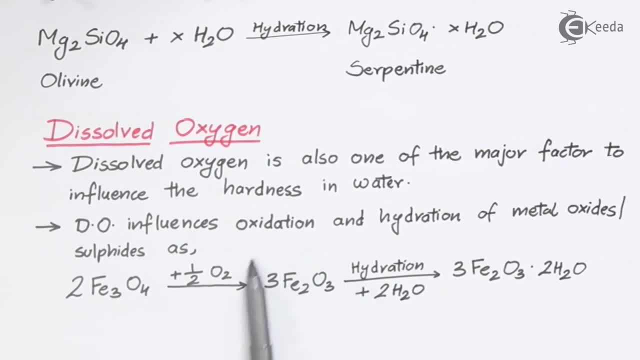 in water, it oxidizes certain minerals to form certain reactants. These reactants then, on hydration, form salts which get dissolved in water, thus converting pure water into hard water. These reactions are the worst kind of reactions, because they not only convert the pure water into hard, 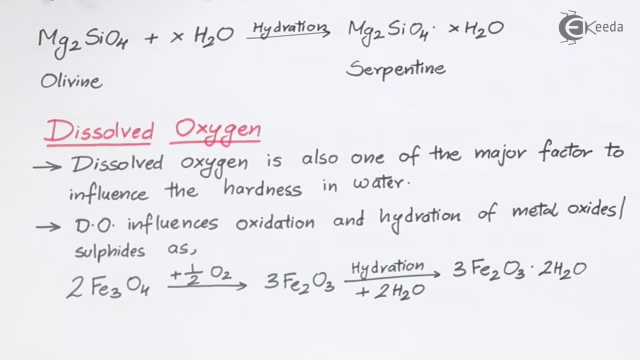 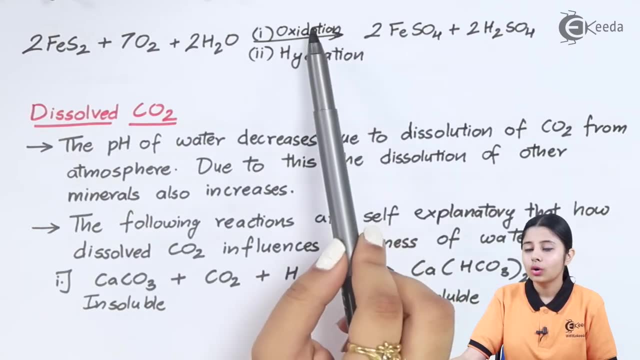 water, but they also eat up the dissolved oxygen which is present in the water. Let's look at one more reaction which is similar to it over here. I have just written it as one reaction, with one arrow On top we have the number one- oxidation that is happening. On bottom, we have number two. 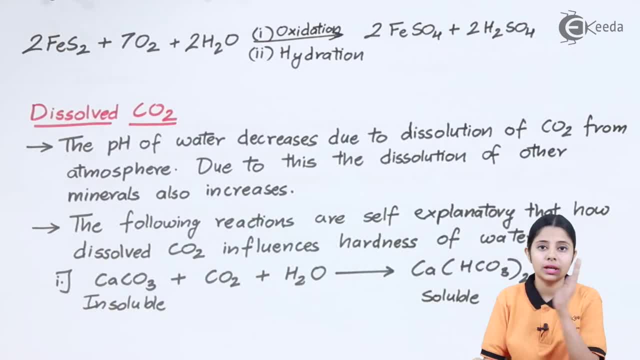 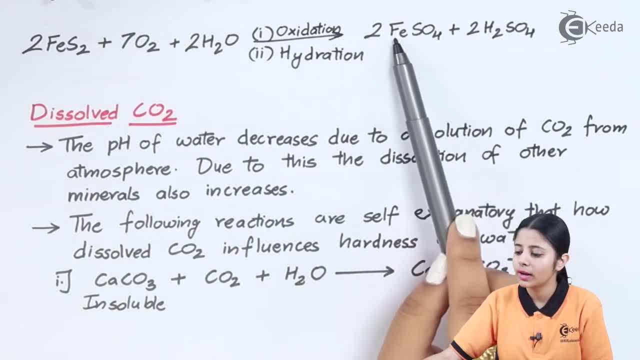 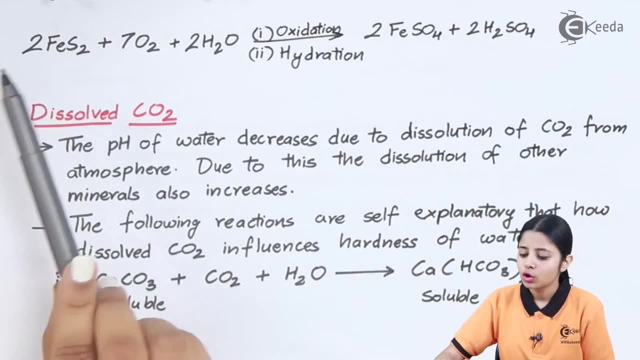 7 O2 plus 2 H2O, forming 2 FeSO4 plus 2 H2SO4.. Now let us actually look at the reaction and balancing of it. So over here I have 2 Fe in my entire reactant side. It's only 2 Fe. Let us look. 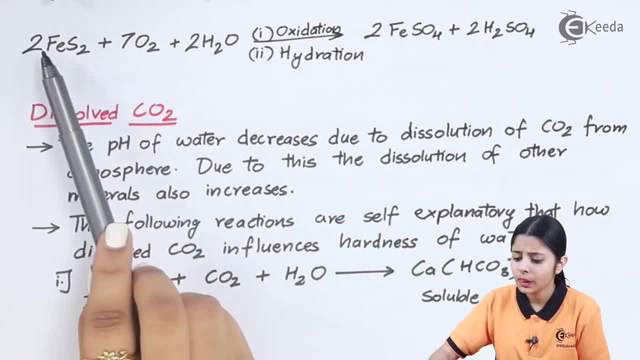 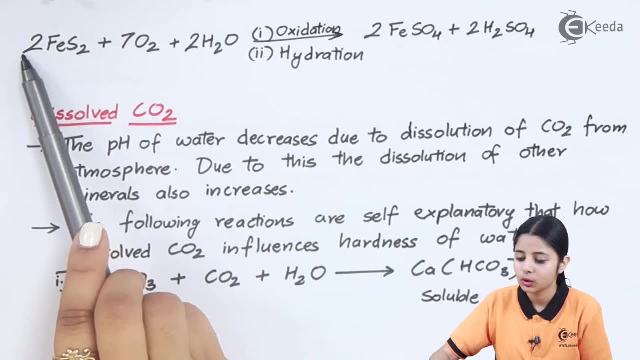 at the product side, It is again only 2 Fe. The number of S over here is 2 into 2, that is 4.. This is twice and that is also multiplied by 2, that is 4.. Over here let us look at sulfur. This is 2. 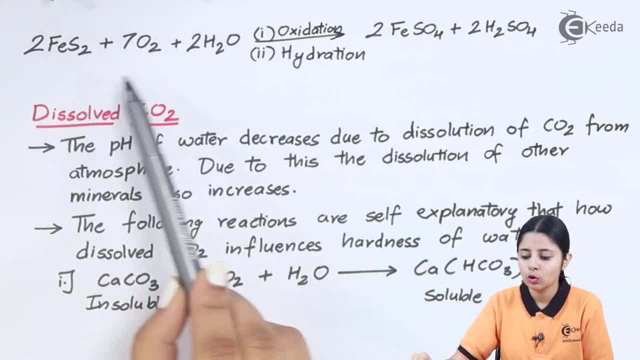 into 2. that is 4 sulfur Over here on my reactant side there is no more sulfur. Let us look at the product side. Product side: I have 2 over here and 2 over here. that is total of 4 sulfur. So even my 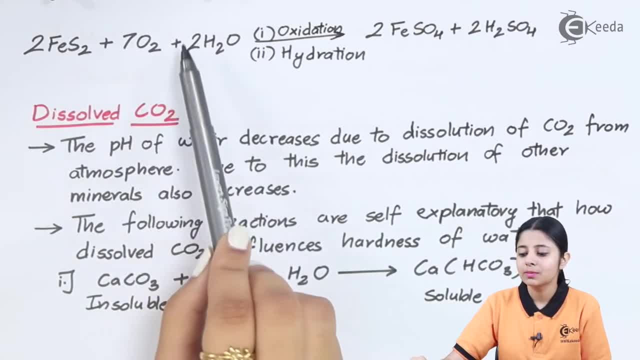 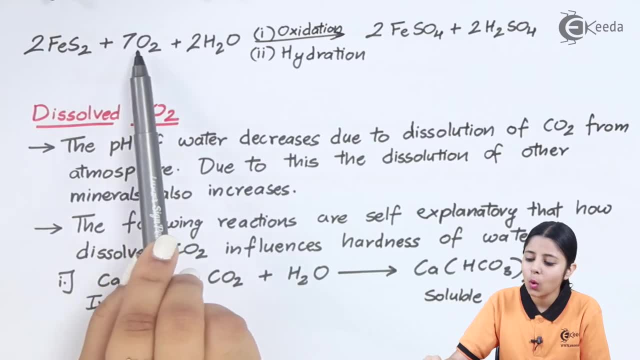 sulfur is balanced. Now the most important part of balancing is balancing of oxygen. We can see many oxygens on the reactant side and many on the product side as well. Let us see I have 7 O2. that is O2 into 7. that means twice of oxygen into 7.. So 7 into 2 is 14.. 14 over here plus 7 into 2 is 14.. 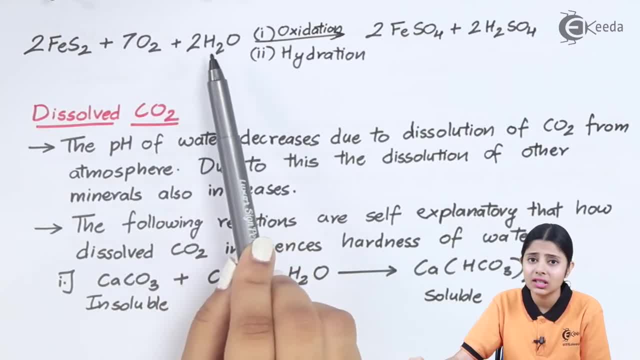 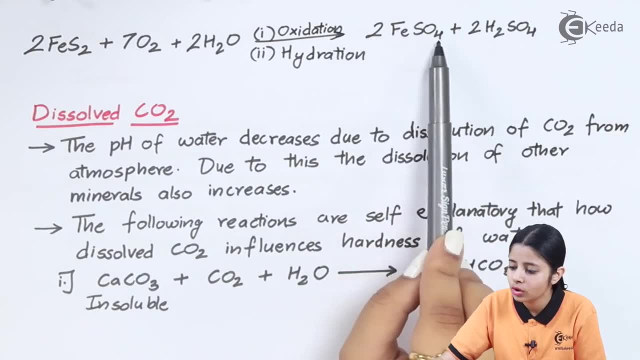 14 plus 2 H2O. So 14 plus 2, that is 16.. I have 16 oxygens on my reactant side. Let us see the product side. On product side I have O4 into twice 4 Tusa. 4 Tusa is 8.. Over here I have H2SO4 into 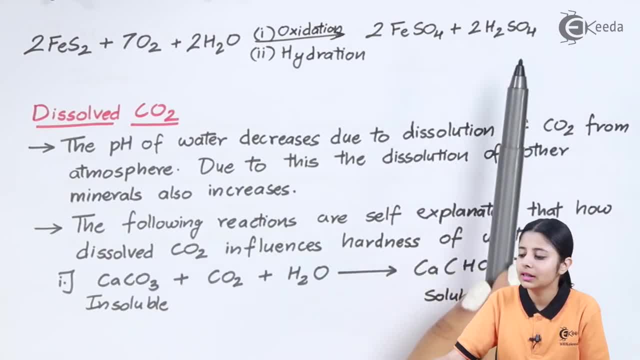 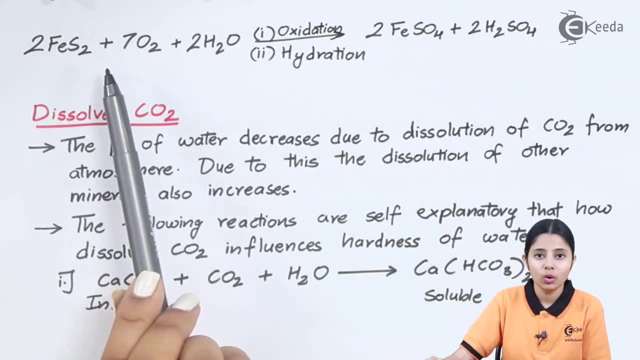 twice Again over here: 4 Tusa, that is 8.. So 8 plus 8, that is 16.. Over here we have 14 plus 2, that is 16.. Over here we have 8 plus 8, that is 16.. So overall, over here we have 16 oxygens on the reactant. 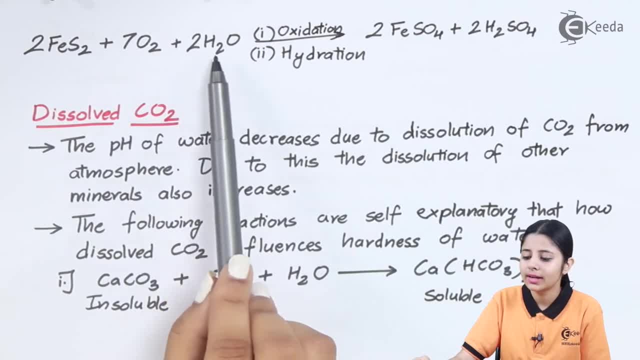 of product side. Finally, we balance out the hydrogen twice H2, and that is also twice Over. here also H2, and that is also twice. So this oxidation hydration reaction of mine is completely balanced. Moving on to dissolved CO2.. The pH of water decreases due to the dissolution of CO2. 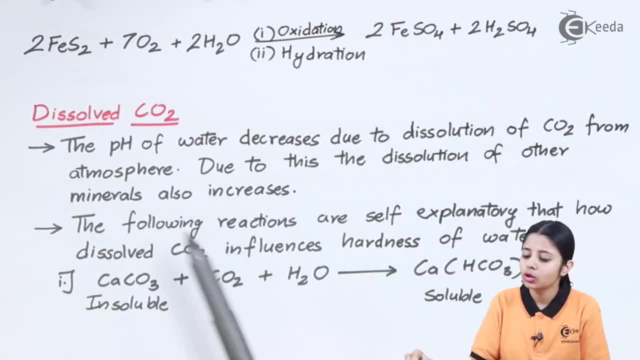 from atmosphere. Due to this, the dissolution of other minerals also increases CO2. itself is an impurity, but that is not it. It also enhances the other impurities to be in it and get dissolved in it. That is the reason why CO2 is one of the major factors. 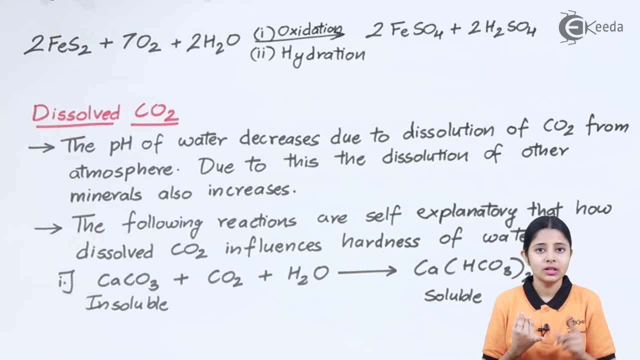 influencing the hardness of water. It itself gets dissolved. It itself disbalances the pH of the water and apart from that it also enhances or supports other impurities to get dissolved in water. The following reactions are self-explanatory: that how dissolved CO2 influences hardness of 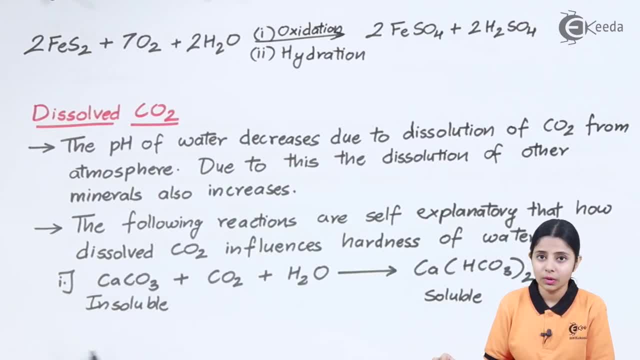 water, So I have CaCO3.. The CaCO3 is insoluble in water, but since the water I have contains CO2, that is the reason why I have written this. So this is the reason why I have written this. So I have written CO2 plus H2O. CO2 plus H2O is nothing but CO2 dissolved in water. This CO2 plus 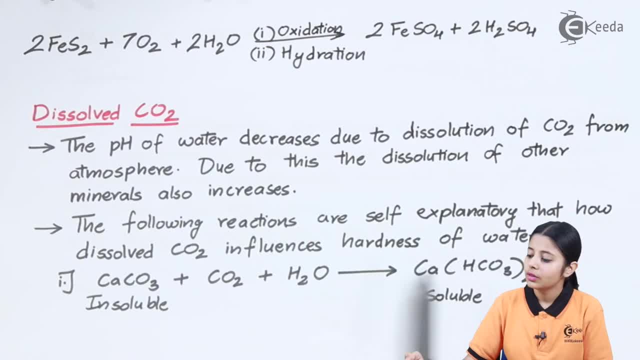 H2O forms CaHCO3 twice. Now this is soluble in water and that is the reason why the calcium, which was insoluble before, has now become soluble and a part of water, leading to impurity of water. Let us see the balancing of this equation. We have CaCO3 plus CO2 plus H2O on my reactant side. 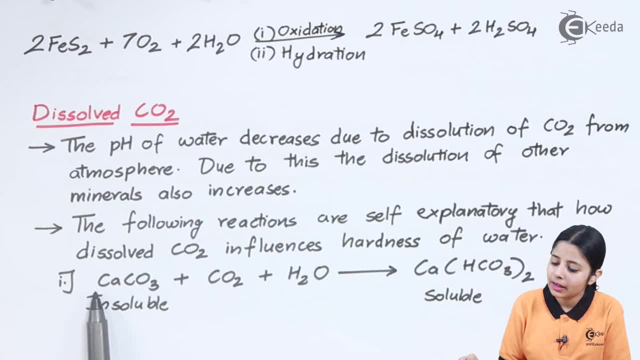 Let's take one, one element at a time. Let's start with calcium. I have CaHCO3 on the reactant side. Ca is one Over here. I don't have any Ca Over here. I don't have any Ca On the. 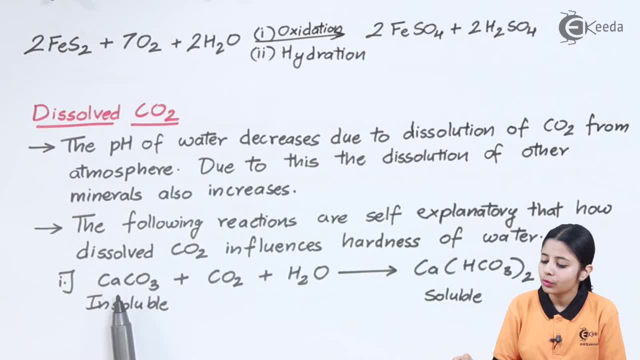 product side also, I have one calcium Over here. then, looking forward to carbon, I have one and two, Two carbons on the reactant side. Over here I have carbon. that is twice two carbon on the product side. Let's see the number of oxygens over here: O3 plus O2 plus O, 3 plus 2, 5 plus 1, 6.. Again O3. 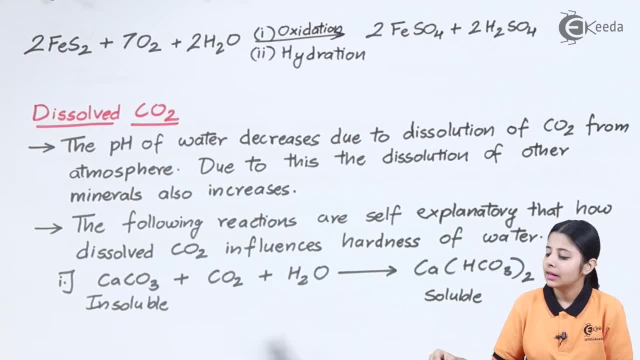 5 plus 1, 6. 6 oxygens are there. Let us see: on the product side this is O3. twice, That is 3. oxygen twice, That means 3 into 2, that is 6.. So on my reactant side I have 6 oxygens On my product. 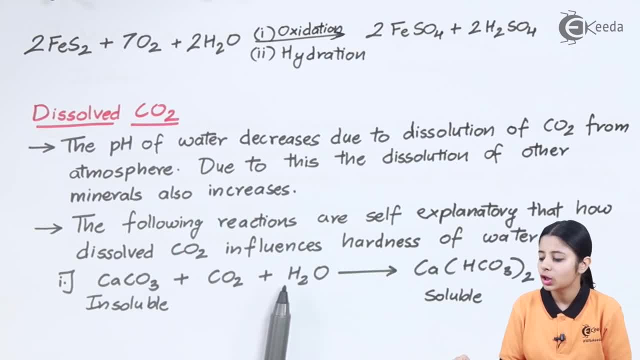 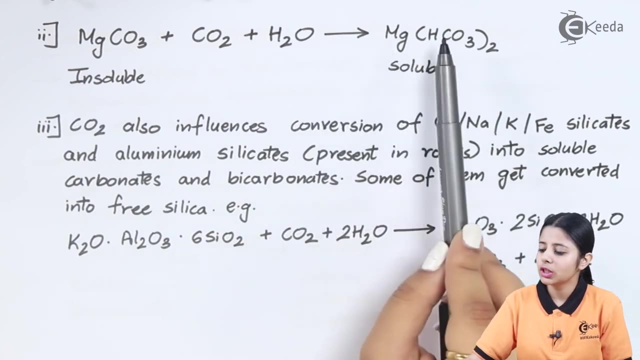 side I have 6 oxygens Moving ahead with hydrogen. I have 2 hydrogen, over here H2 and over here also I have hydrogen twice H2.. That means this is a balanced reaction. Let's look at one more reaction: H2 forming MgHCO3 twice. This reaction is exactly same as the previous reaction, but in the previous. 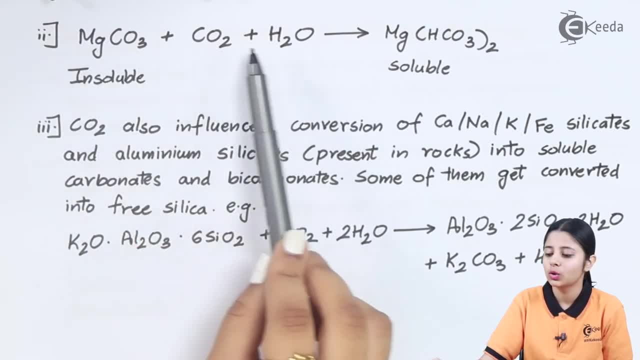 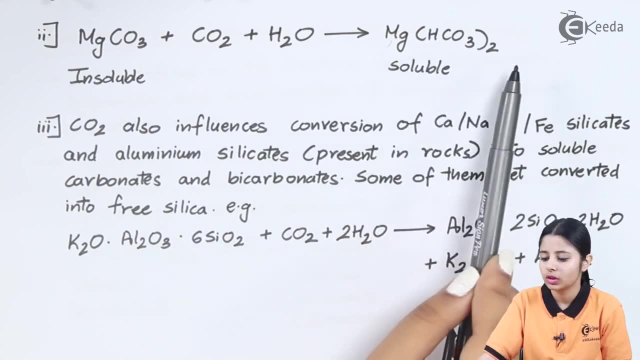 reaction: instead of Mg we had Ca. We had CaCO3 plus CO2 plus H2O, forming CaHCO3 twice Over. here we have MgCO3 plus CO2 plus H2O, forming MgHCO3. twice Again, MgCO3 is insoluble, but with the help.